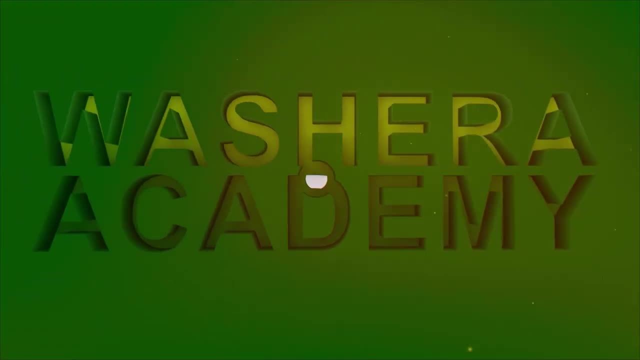 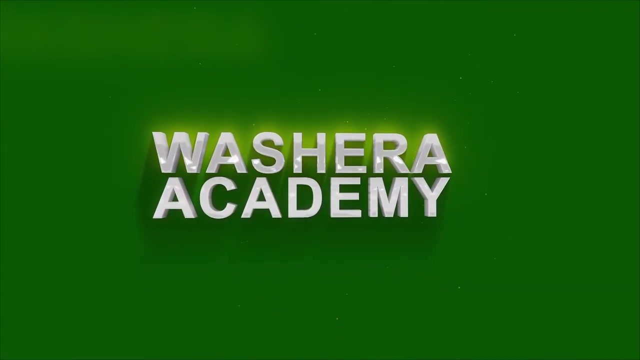 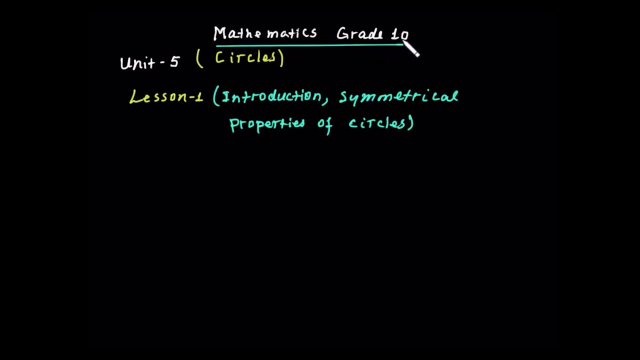 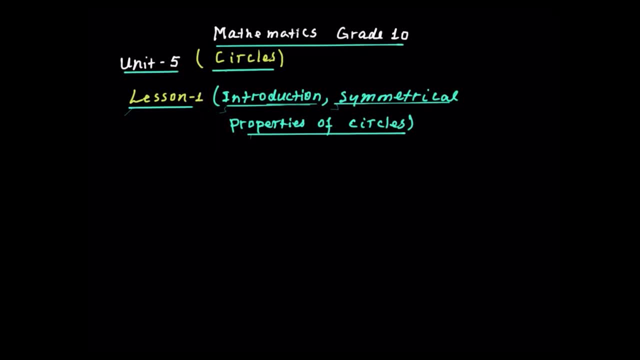 Symmetrical Properties of Circles. Explain Madrake. Use the Symmetrical Properties of Circles to solve related problems. At the end of this unit, write Angle Properties of Circles in their own words. Apply Angle Properties of Circles to Solve Related Problems. Apply Angle Properties of Circles to Solve Related Problems. 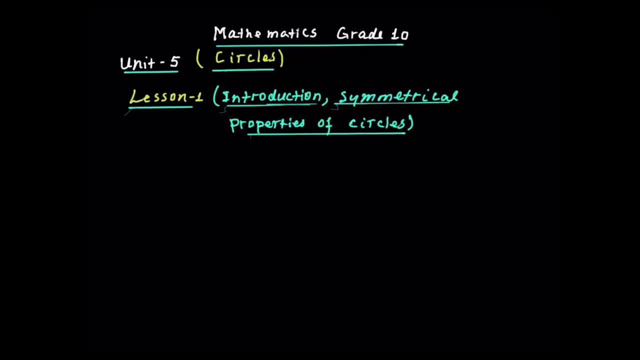 As an introduction, you have learned several concepts and principles in lower grades of circles. Circles are important to understand. Let's start, Let's start, Let's start. In this unit, we will learn more about Circles, Parameters and Area of Segments and Sectors of Circles. 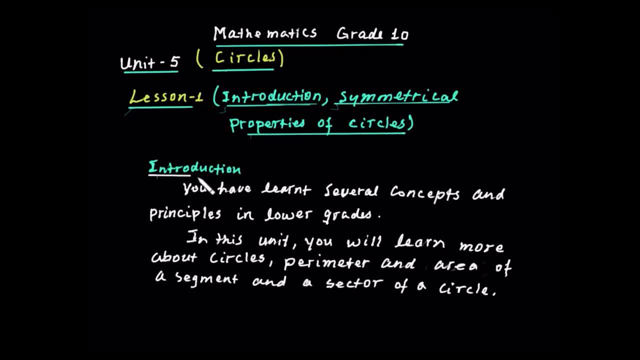 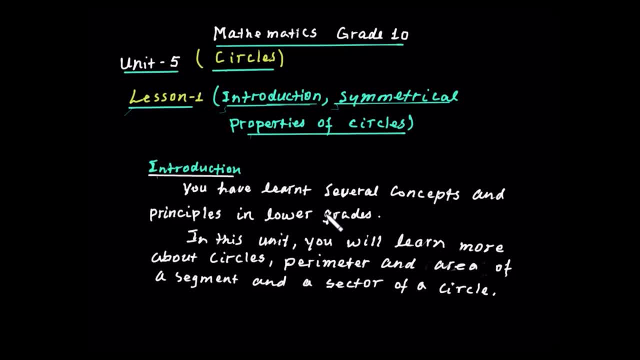 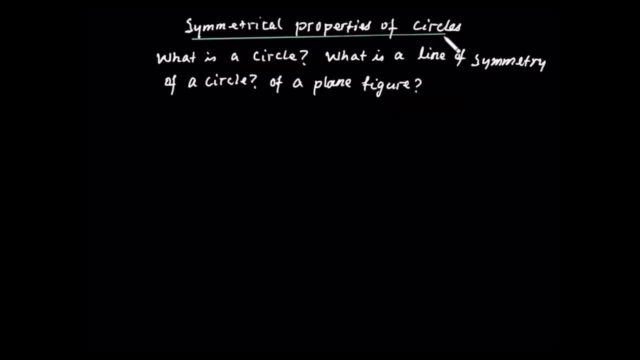 Let's start with the Symmetrical Properties of Circles. What is a circle? What is the definition of a circle? What is the line of symmetry of a circle of any other figure? The definition of a circle in the קτ, essereerdings of a circle is: 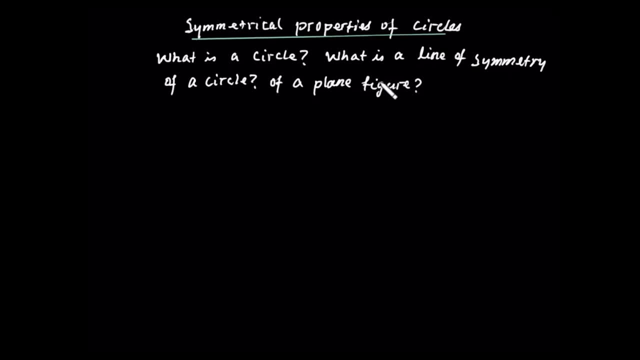 The line of symmetry of any plane figure, and especially of a circle. What is the name of a circle? What does a circle face? If you know the answer, you can say it in objectively, But you will not be able to answer straight from there. 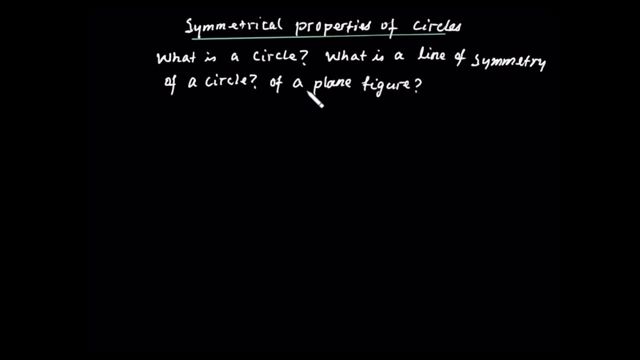 So what is the definition of a circle? another go is simply set of pointers in a plane which are equidistant from one fixed point. So this is the definition of a fixed point. The definition of a fixed point is a circle is simply the. 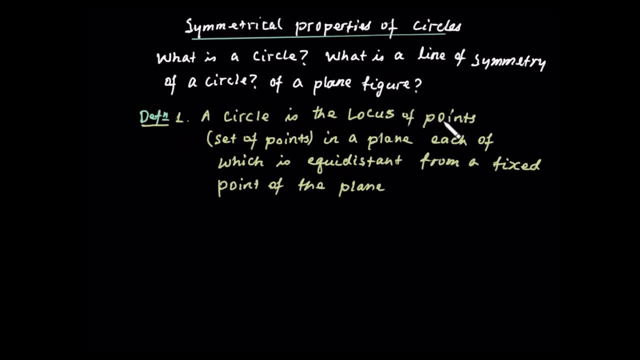 locus of pointers. Locus means the set of points. Set of pointers in a plane which are equidistant from one fixed point, Each of which is equidistant from a fixed point of the plane. Set of pointers in a plane which are equidistant from one fixed point. 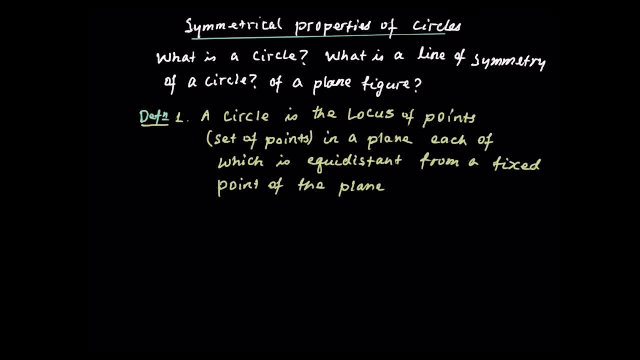 This is called a circle. The definition of a fixed point is: a circle is a locus of pointers. Now let us see how to identify a surface point of eachrijitoriel. So for each location, one observedPlease follow the given shr arrow. Please follow the sameつth equation. 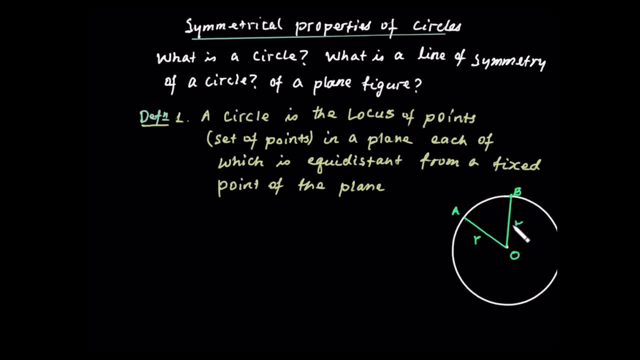 Now we must find the surface point of eachrijitoriel. So to find the surface point of eachrijitoriel, We need to find radiations in a spr���りましたasis, So to see the radius of eachrijitoriel, the distance from O to any point of this has the same distance in normal manner. 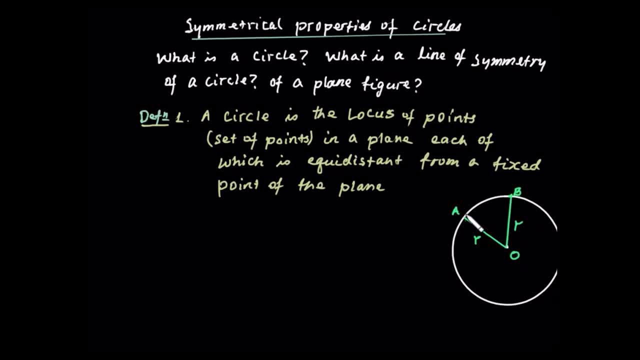 So we could stand to be below. yeah now. So let's say two points now, Circle In English on fixed point, one center of the circle now. So let's say usually circle, The salient circle, circle O. 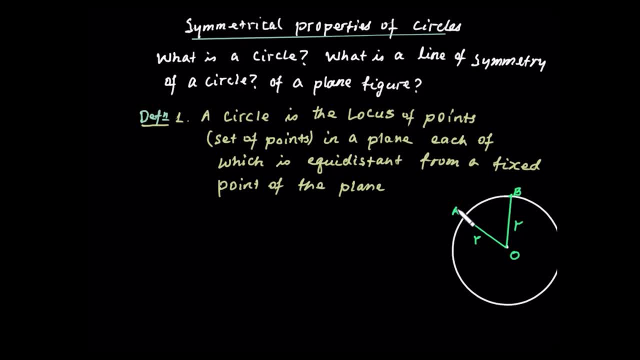 The fixed distance is called the radius of the circle. So O, A, O, M, O, B, We call it the radius of the circle, And usually it is represented by R. Okay, let's see this now. The fixed point is called the center of the circle. 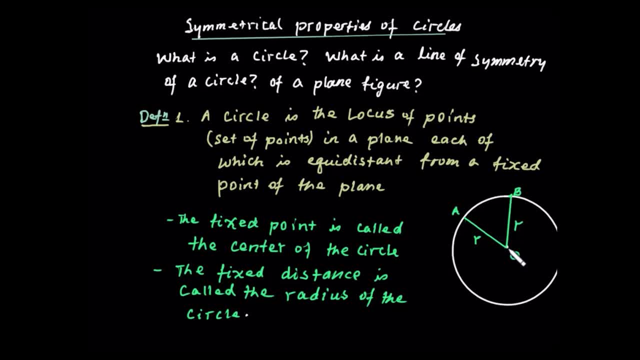 Let's see the center. The circle is the same, but the center is different. The salient circle, circle O. So the fixed distance is called the radius of the circle. This is the fixed distance because all the points are the same. 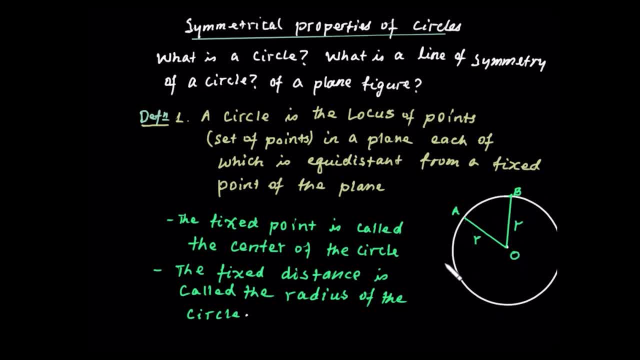 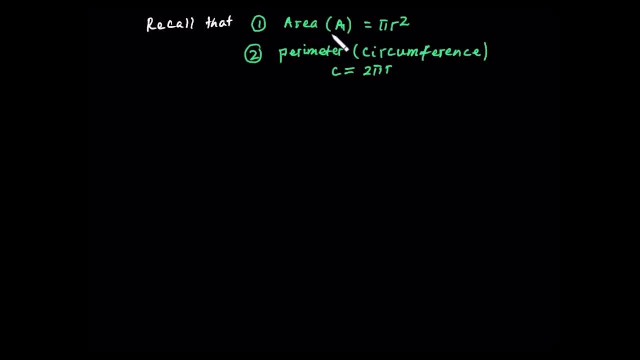 They are equidistant from this point. This is the point we have to see. What is the circle? This is the fixed distance, what you can call radius. So according to the law of law, it is written that the area of a circle 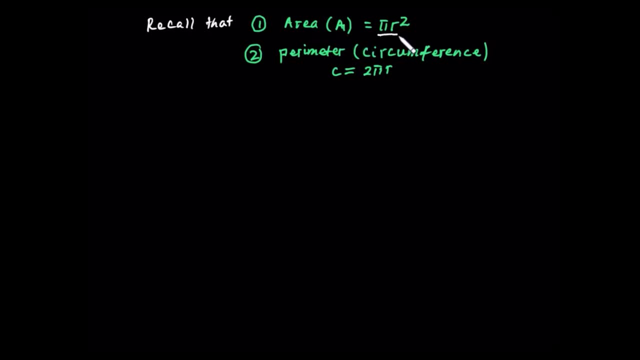 is also called Aspire square, and its shape is a perimeter or circumference. The circumference of a circle is usually C is equal to 2 pi r. This is the formula. Now let's define the line of symmetry. What is the line of symmetry? 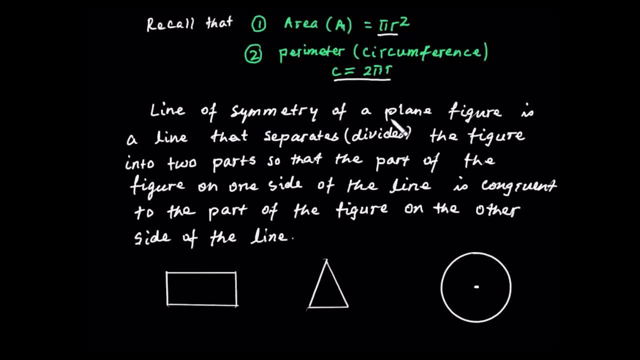 The line of symmetry is not a circle, It is a line. It is simply a line that separates or divides the figure into two parts. The figure is divided into two parts So that the part of the figure on one side of the line is congruent to the part of the figure on the other side of the line. 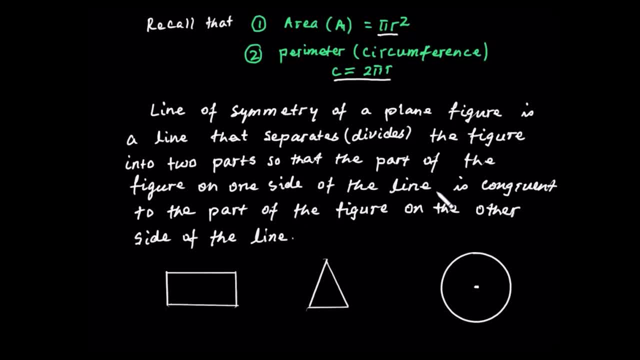 So this line is a figure divided into two parts. It is a line that divides, or divides the figure into two parts. It is a congruent figure. Now let's see a few figures. This is a rectangle. This is a rectangle. 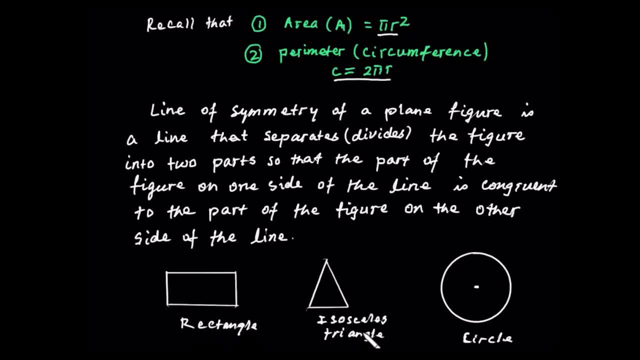 For example, if you have a line of symmetry, for example, a rectangle. in this case, if you have a line of symmetry, you have to find the congruent part of it. If you have a line of symmetry, if you have a diagonal line, you have to find the congruent. 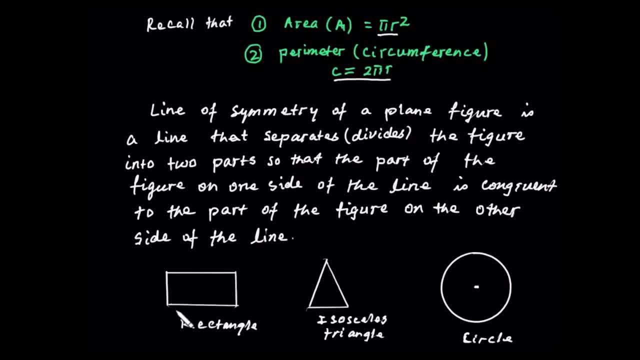 part of the sum because you have to have the congruent part of this line. So you find the vertical coordinates in accordance to the congruent part. If you have a horizontal line, you find the coordinates and you will be able to untukune it. 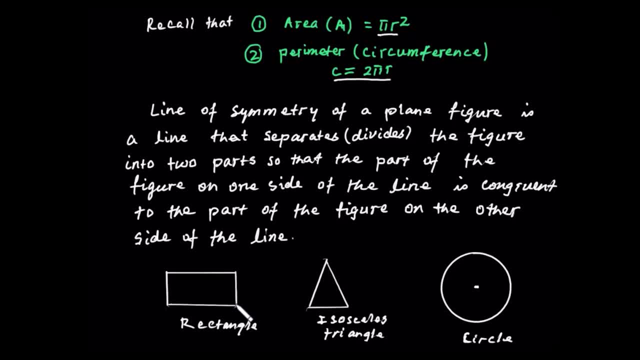 Of course you will be able to use this line of symmetry. It will be a straight line By Briева's method. you can use this line of symmetry, symmetry. last night you let us all in rectangle, this barring where you call a mama, kind of the coverage, but Greg, but cool, and on the back and you were cool. 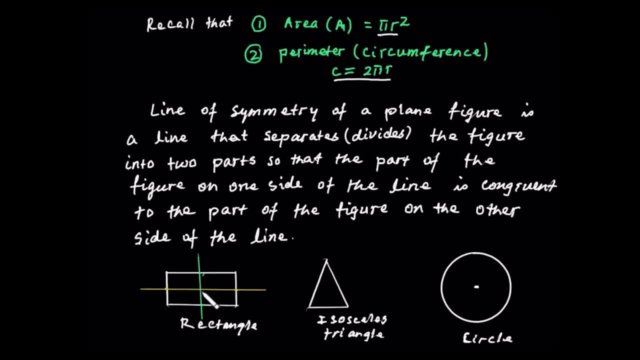 and low the catamar. so the CNN Adelaide, each in your center of the rectangle, not each point mother. no, you will have to. McGonagall agree, but I was. I say I saw. so let's triangle and the line of symmetry be channeling or original one. 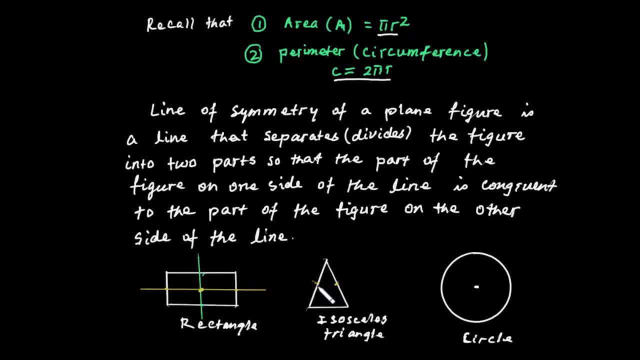 as well as two sides coca-cola. I sell a set of allah, but two sides of a triangle are equal. no, so let's in this. you could call you, and this is me, got the mood but got the time I'll. I'm gonna cover the nobody ever take, so I'm not going that. 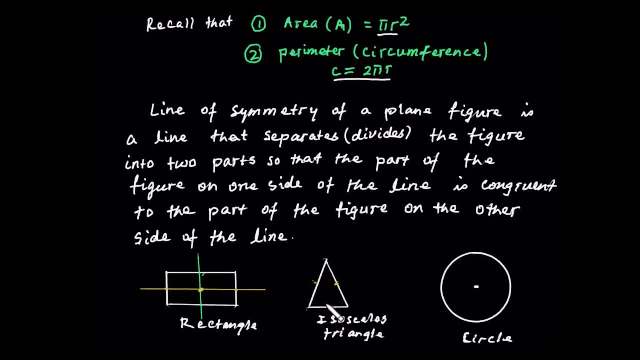 but nothing, I'll, I'm, I'll, let me cover low is a line of symmetry. so let's see, isosceles triangle has exactly one line of symmetry. and you know, last night let me tell you, a line is a line of symmetry for an isosceles triangle. okay, 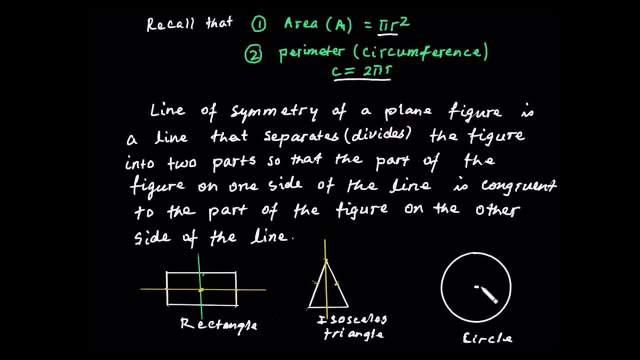 circle is a net, a little cool, what I'm a couple of percent or email line. this line separates the circle into two arcs: the arc and the arc. no, young and work. some circle, no good, my salon. so let's see nasula to congregate in a channel. but I 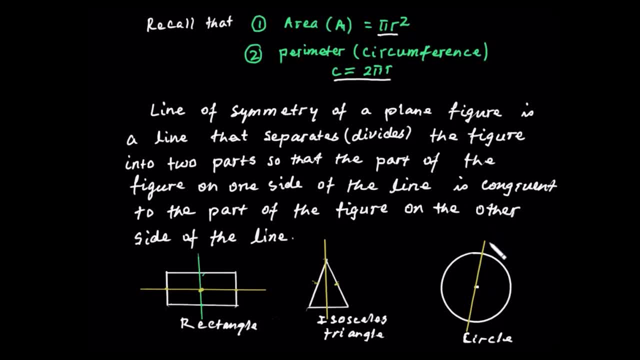 know I'm a kindness and not fat Joe, you got a man, so let's see one now. line of symmetry: me ballot. and as the line which not many young line, through the center of the circle, divides the circle into two parts, the MN does under simple cover, this line is also a line of symmetry, snow line of symmetry. 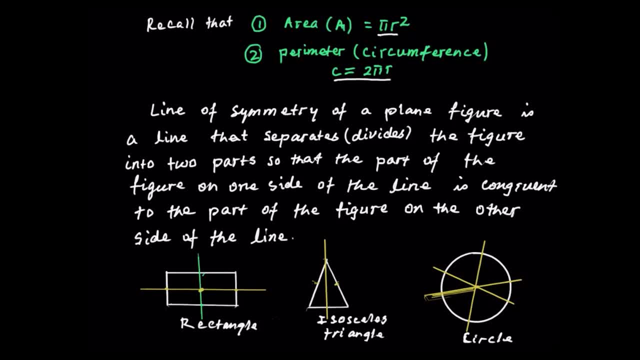 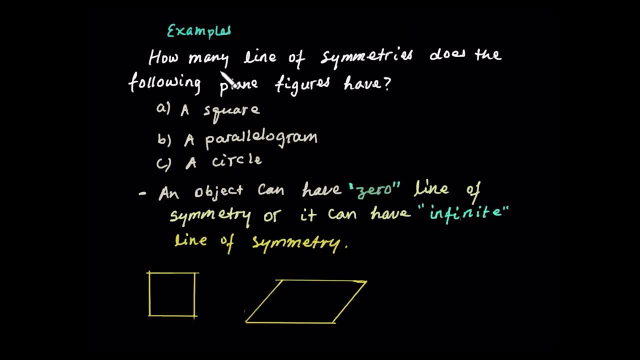 ini, botbard, gotta is t, and then BI coaching Lizoo presenting the example. would a teacher saber, Okay, organiz, is the growth course. family line of którzy. karempi language: is you like a bringer? allah, okay, alreza, square. you know something? is you deformation squaring? well and a ya, yeah, rightOG at now fromOLU. they're gonnaCome on out outside. I'll be here in about internet news. you look it out and the example. what does that meanre planes to molten's eSo, that's the same. you're looking off to natovising one. the example is consolidation engine. you look at it's in line. you look at it's in line. you culture center. it's an originalankiiran. we're gonna use sign that doesn't fall at bay. parking次 du. 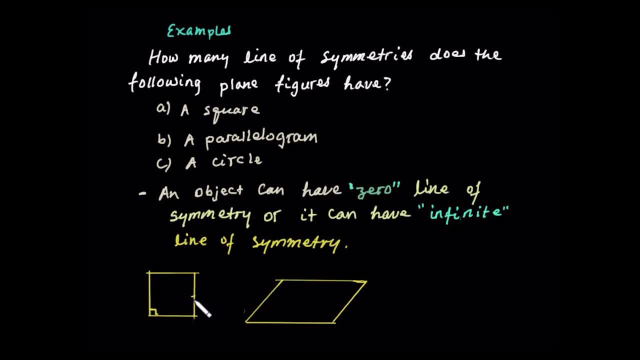 and then, yeah, yeah, right angle. now formula the ganara to congruent ratio. resist query: mess below. you know, all the interior angles are right angles and all the sides are equally links. yeah, no, square man. so as the sent line of symmetry. yeah, layman's lateral. now tamil kato in the. 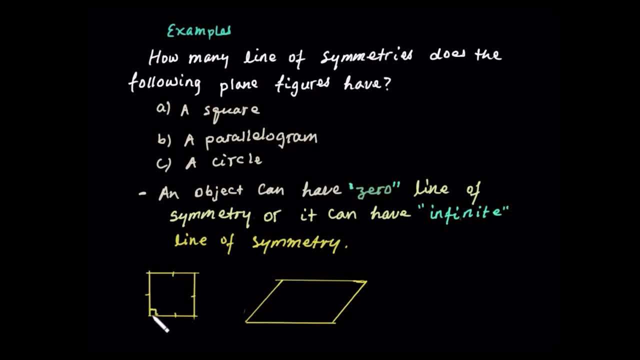 line of symmetry which, and then yeah, but nasi, diagonal trauma, kind of a couple. here is the libid era America, two segments lighter value segments later about, so that the wild line of symmetry on busy- no, I'm not in that in the zoo- another line of symmetry. vertical in the seven water, another line of symmetry. 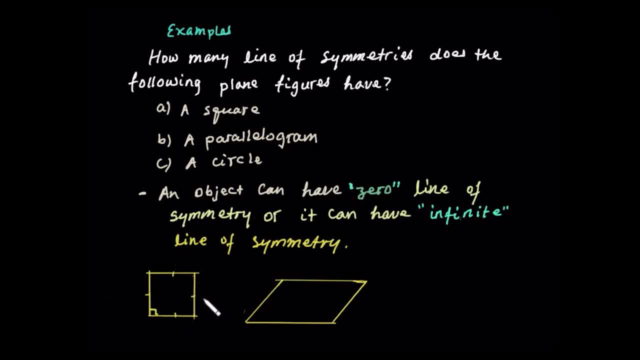 horizontal, in the zip of blood, another line so that the arad line of symmetry, in order to know nasi muba, bigger lasso, okay English. in the ziarah line of symmetry, a low square, parlogram, license head, a parlogram palal oposites are parallel now. 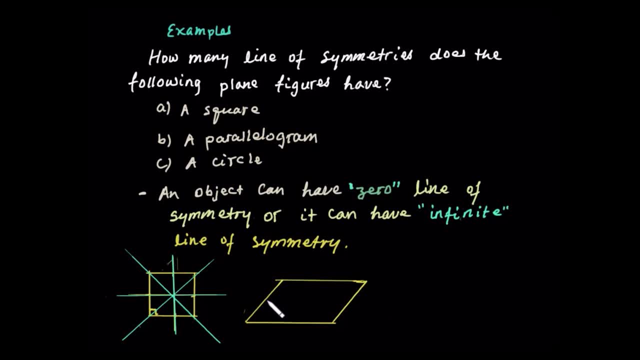 yeah, because the car parallel a because the car parallel so that the sense line of symmetry- you know, rich lal, no painting all. I am a kind of no, but yeah, when I look to my kind of the not for got a malino gnatum, yes, I think, as 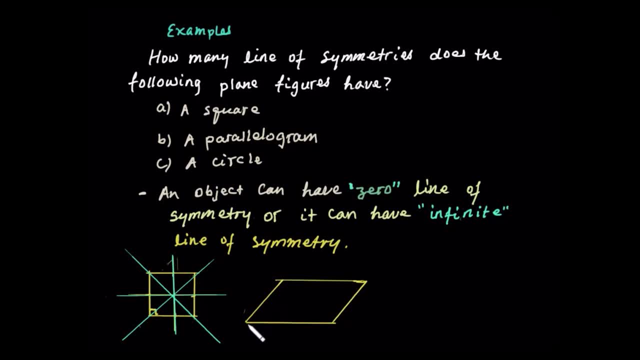 the side car congruent slalom or a monotone slim manner got get busy. I'm a kind of the not for you here is the line literature and as you busy side American, but not for him the line literature. so let's see diagonal to line of symmetry. you know it's room for a parlogram cuz under the vertical you. 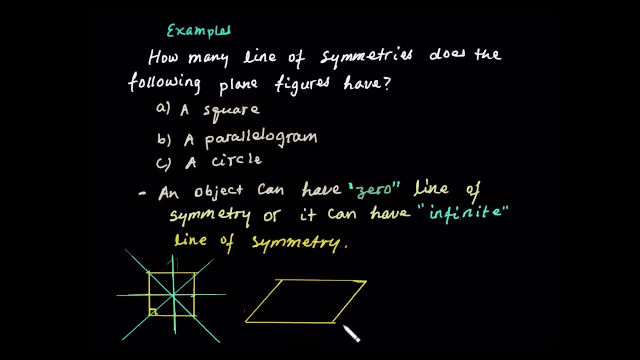 know, and the gym before tour, when Monday's the end, and burness the parallel on Allah and the seemed courted A�O lacu legata. material: lemon polio Amachan. citata for the zien 몇. our motto, Matt al-alazi: a parlogram has no line of. 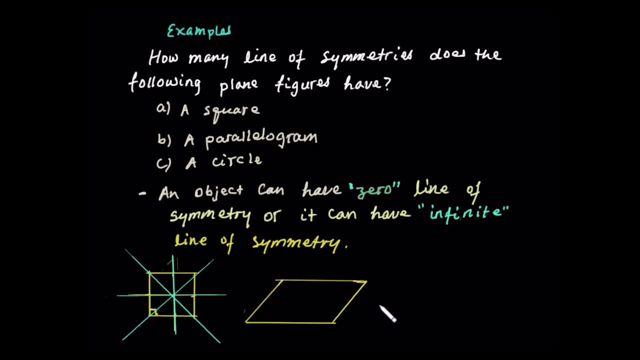 symmetry: horizontally record 1. Saturday's not on site of the line when append down of the line got lit. figure are part of figures, the gun onion each. So a parallelogram has no line of symmetry. A circle has many lines of symmetry. A circle has many lines of symmetry. 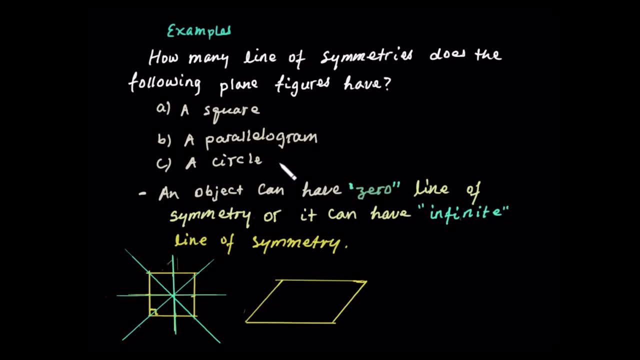 Any line through the center of the circle is a line of symmetry, So we need to find the line of symmetry. A triangle has one line of symmetry. A rectangle has two lines of symmetry, So we need to find the line of symmetry. 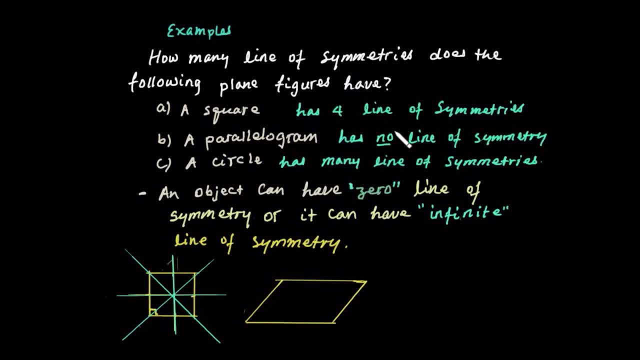 A parallelogram has no line of symmetry. We have a question here. A square has four lines of symmetry, A parallelogram has no line of symmetry at all, And a circle has many lines of symmetry. So we have a question here. 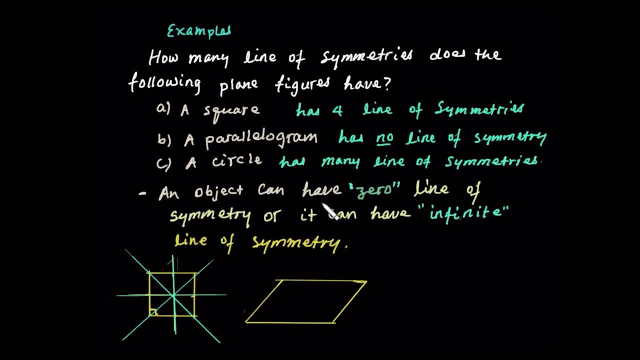 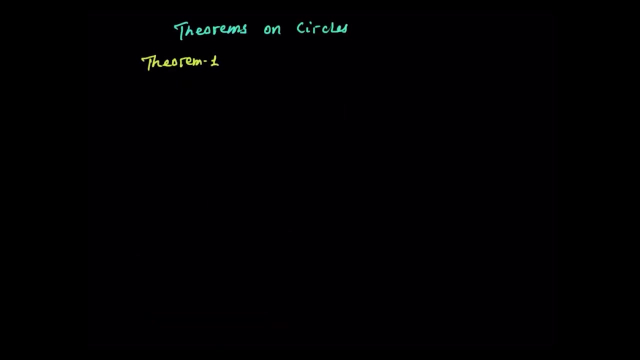 Does a figure have zero lines of symmetry? No, Look in the parallelogram line of symmetry and the plane figure or it may have, or it can have infinite line of symmetries, just like a circle. This is the net watch, and now we will see theorems and circles. 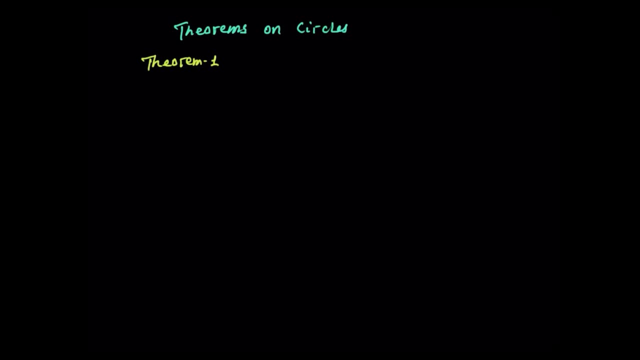 So let's see the theorems and circles. Let's start with theorem one, the first theorem. Let's have a look. The theorems and circles. Let's start with the theorem: The line segment joining the center of a circle to the midpoint of a chord. 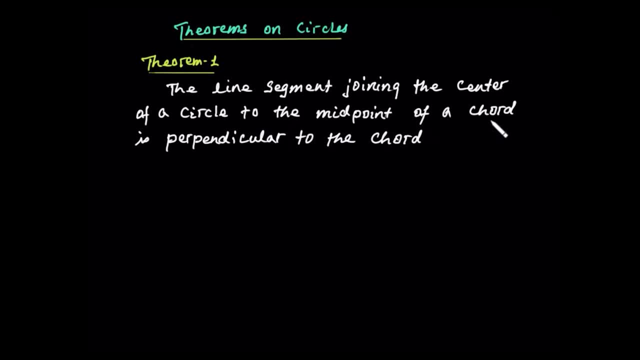 The chord is the middle point of a circle. The segment joining two points of the circle is perpendicular to the chord. Let's have a look. The theorem, The theorem which, in geometry, proofing another gotcha on it, Marra gotcha on it. 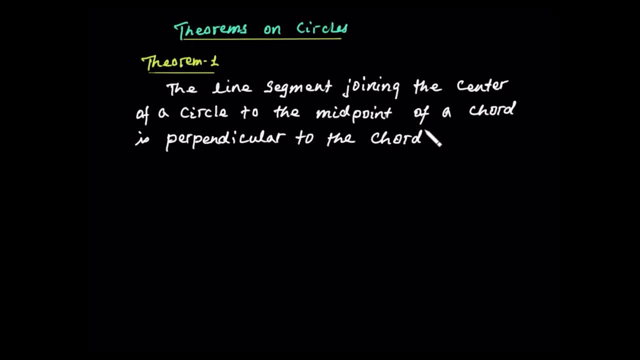 It's fact Fact on it, But we need to prove them. So let's see The theorem. Marra gotcha on it. You know what I'm saying. So let's see Here. let's see By figure. here let's see: 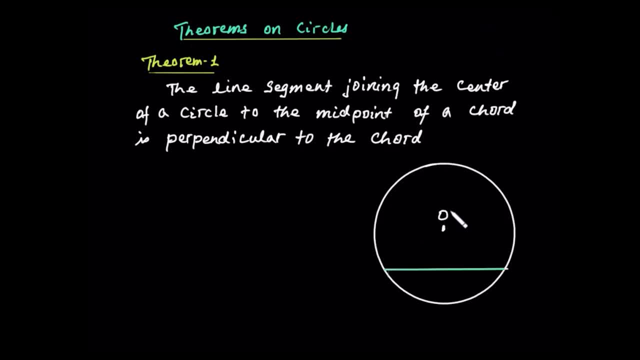 The image of a room. proof, Let's have a look. Let's have a look Here: circle on it, The center of it. O on it, Because the center of the circle is O and it represents another chord. The chord is a segment joining two points of the circle. 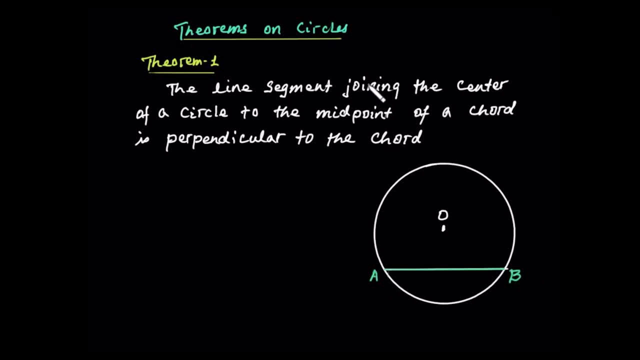 For example, this is chord A B, The line segment joining the center of the circle. This is the point To the midpoint of the chord. The chord's midpoint is the same. This is the midpoint M. So let's see. 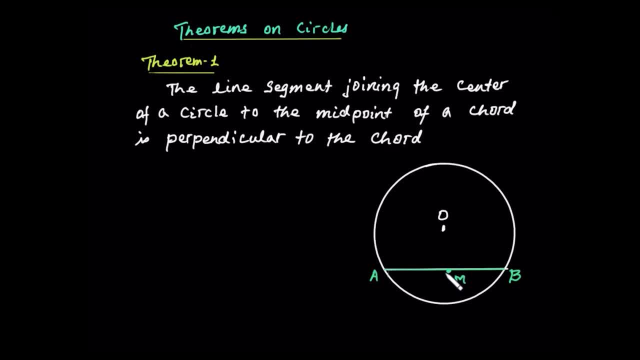 So let's have a look. Let's have a look Here. the line is perpendicular to the chord, So this is the right angle Here let's have a look. So let's have a look at the proof. 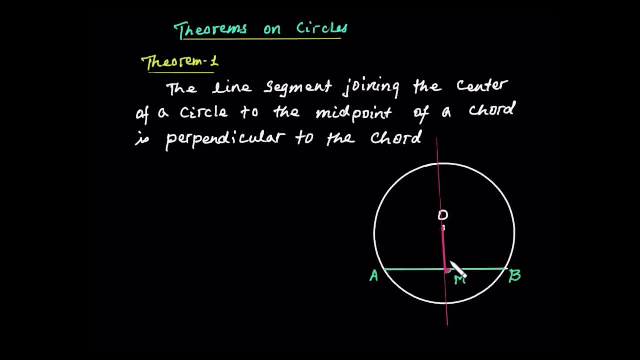 Right angle, Perpendicular, It's not right angle. So let's have a look. So let's have a look at the proof. So let's have a look at the proof. So let's have a look at the proof. 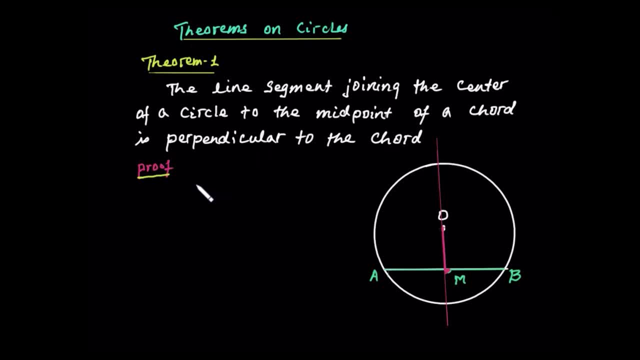 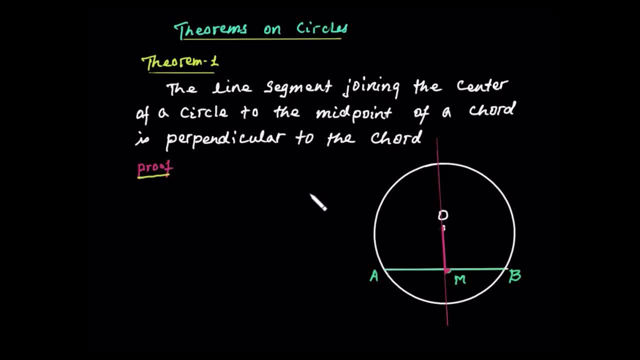 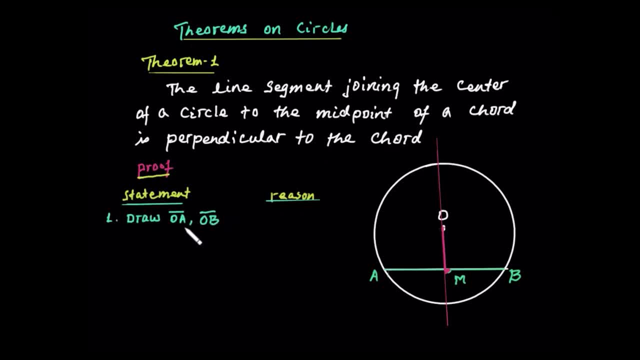 So let's have a look at the statement and the reason. So let's have a look at the statement and the reason. This is the reason why we call it a construction. Where do we draw? I draw OA and OB. This is the radius. 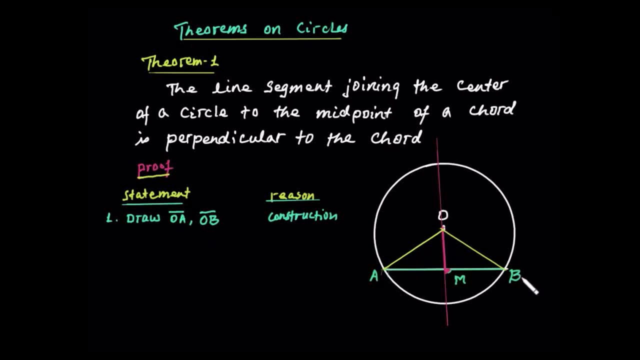 This is the triangle. OAB is the isosceles triangle. This is the isosceles triangle. This is the line, This is the point. This is the triangle. This is the equilateral triangle, Because triangle OAB is isosceles. 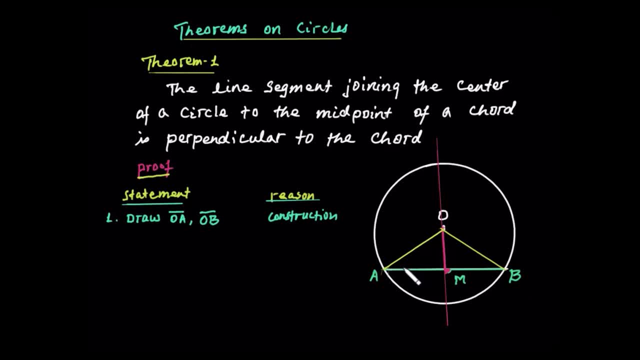 This is the radius. This is the radius. This is the equilateral triangle. This is the second step. This is the line. This is the second step. OA is equal to OB. This is the radius of the circle. AM is congruent to segment BM. 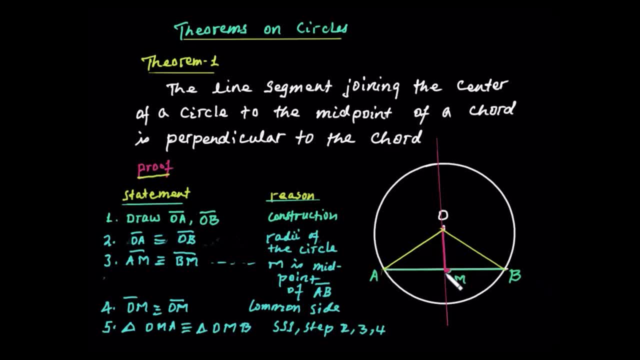 AM and BM are the same. Why? Because M is the midpoint of AB. This is a given information. M is the midpoint of AB. This is a given information. OM is the commune side of the triangle, The isosceles triangle. 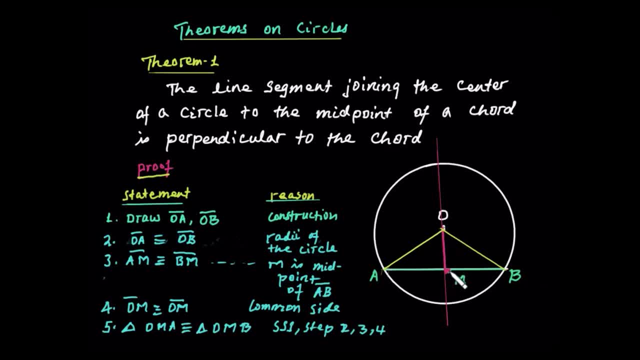 is consecutive with lines. Since this is the middlepoint of the Milky Way, It is called the triangle As perceived flowing along the sides. There is a commacaksın in the am isosceles triangle. This is the triangle. This is the triangle. 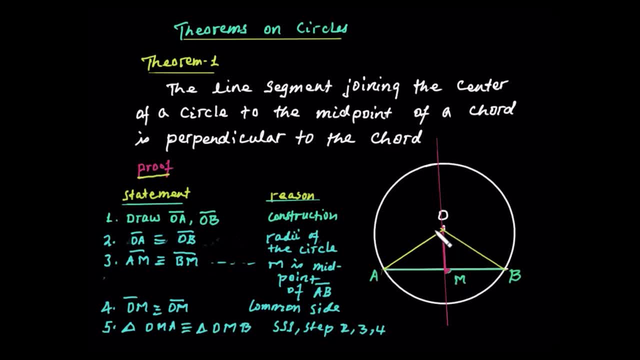 And this is the triangle. There is a triangle side, side side. the two smaller triangles are congruent. Slavich in dit argil traco no Yama jamarau. triangle om a is congruent to triangle om b. no Slavich basanet congruent, yo na allo. 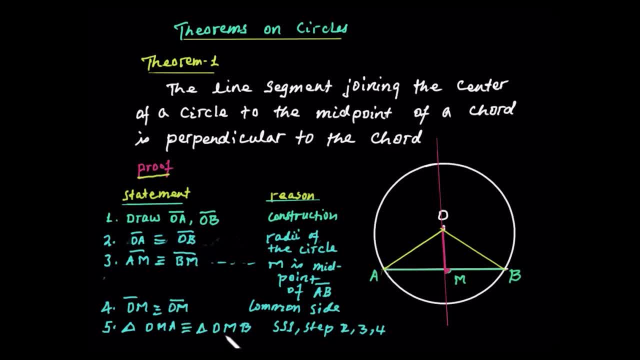 En dem homine gran side side side en enye sostu nacho Slavich by side side side en enye. triangulo congrient nacho Definition of congruent triangles: corresponding angles are congruent and corresponding sides are also congruent, no. 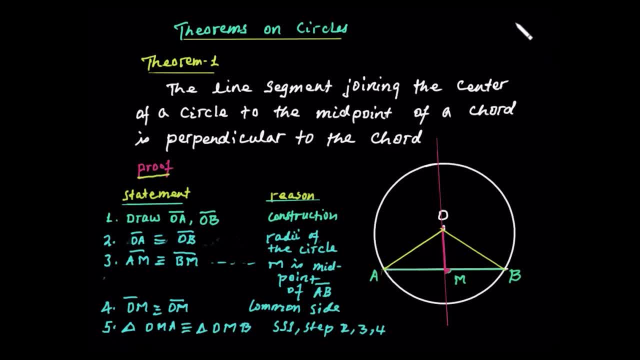 the next page line, we will see the steps. we will see the steps and we will see the angle perpendicular to each other. this is the angle. this is the angle. this is the degree from the first triangle- OMA is the angle. from the second, smaller triangle- OMB is the angle. 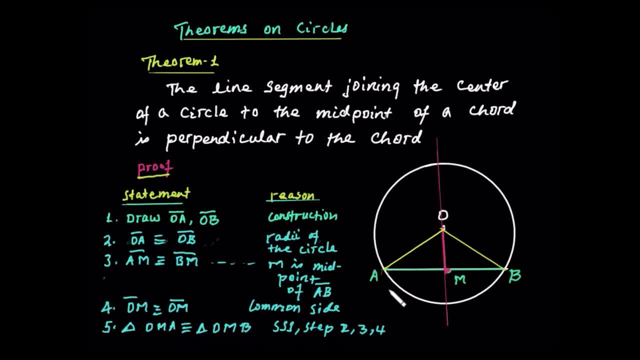 angle. OMA is congruent to. OMA is congruent to by definition of congruent triangles. so this is the angle. this is the angle. straight angle, straight angle. so this is the angle. so this is the angle. so this is the angle the line OM is perpendicular to.